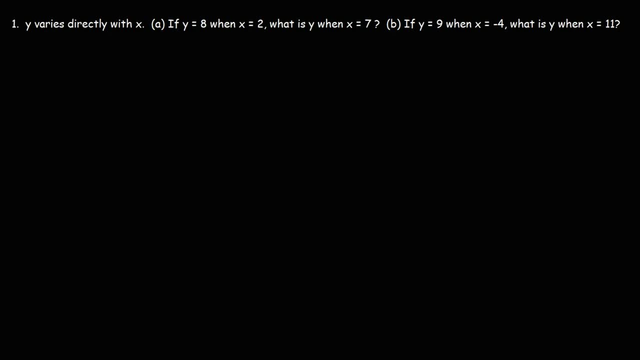 In this video, we're going to talk about direct variation. What is that? Direct variation is the relationship between two variables, in this case x and y. Here's a graph: x is the independent variable, y is the dependent variable. When y varies directly with x, what? 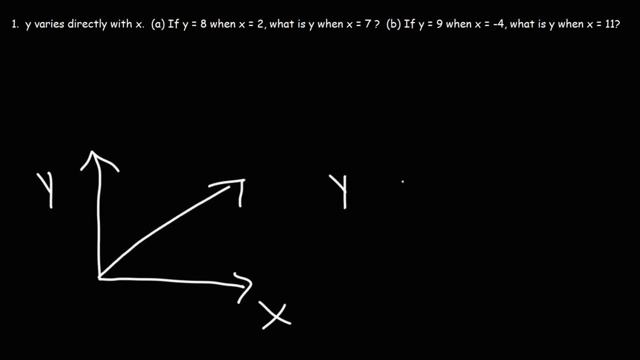 we're going to have is a linear relationship. The equation that corresponds to it is: y is equal to kx. As x increases, y will increase at a proportional rate. k is known as the constant of variation. If you want to calculate k in this situation, it's simply y divided. 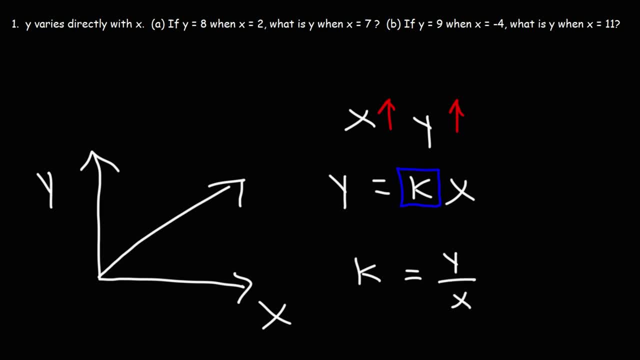 by x. So feel free to write this down, as we're going to be using this information to solve this problem. So let's start with number one. Y varies directly with x. If y equals 8 when x is 2, what is y when x is 7?? So the first thing we want to do, step 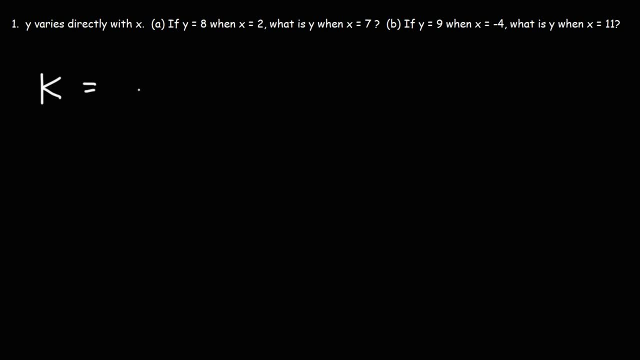 one is to calculate k, the constant of variation. Keep in mind: k is y divided by x. The way this step one can be used is the Driver equation. So the question can be as follows: what is y equal to kx? What is z equal to k? Y is 8.. X equals to actually. 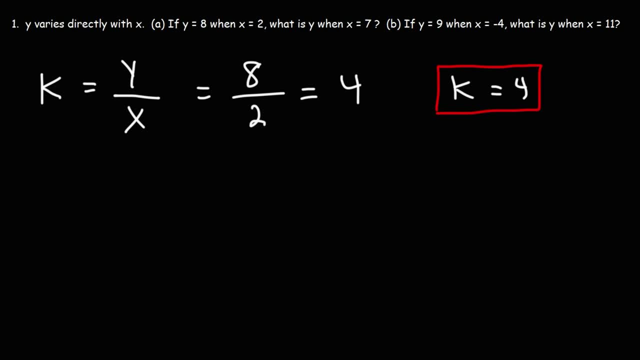 8 divided by 4, so 4 is the constant of variation, So k is 4.. That's the first thing that we want to do From here. we'll use this to calculate y, step one, The second thing that we need. 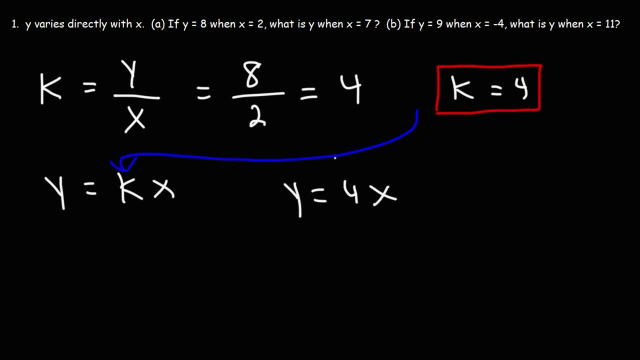 to do is write the equation. Step two화ancalar cherry Wise question. step two is: y is equal to kx. What we're going to do is plug in k into that equation. So the equation is: y is equal to kx. So the formula for y is: y equals 2 of z squared over 2 times x squared. 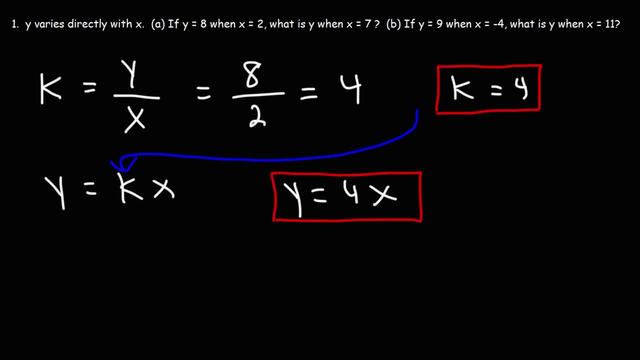 to 4x. Now that we have the equation, we could answer the second part of the question: What is y when x is 7?? So now we need to plug in x. We're going to replace x with 7.. So this is going to be. 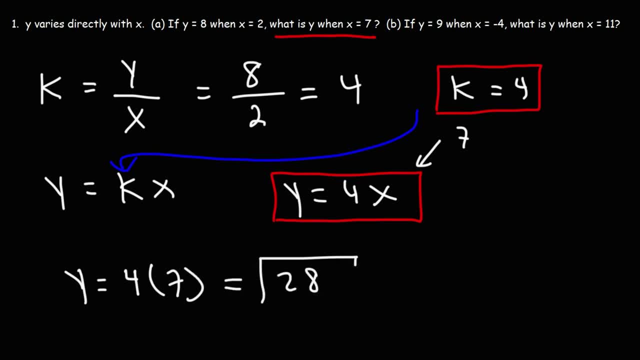 4 times 7 is equal to 28.. So that's the answer for part a, That is, the value of y when x is 7.. Now go ahead and try part b. If y equal 9 when x is negative 4,, what is y when x is 11?? 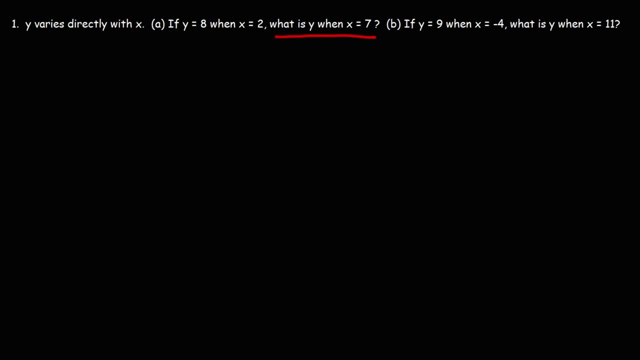 So, step one, we're going to calculate k. Step two, we're going to write the equation. And then, step three, we're going to calculate the value of y. So k is y over x. And then, step four, we're going to 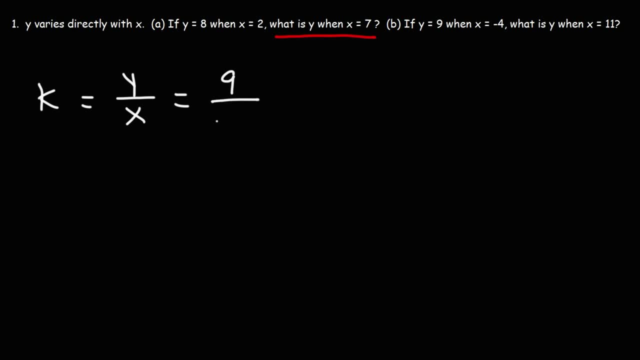 write k as negative 9 over 4.. So now let's write the equation: y is equal to kx. So the equation is: y is equal to negative 9 over 4 times x. Step is to plug in the value of x to get y. 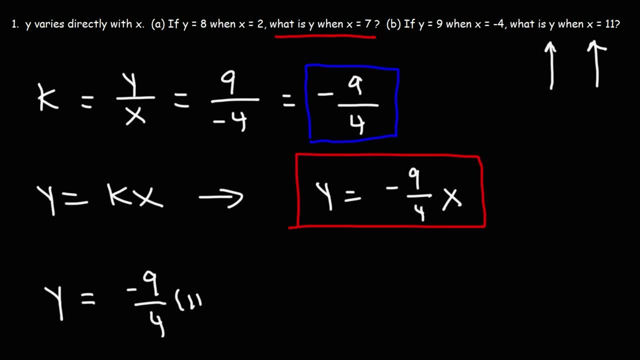 So we want to calculate the value of y when x is 11.. Negative 9 times 11 is negative 99. Now we can't really reduce that fraction, so I'm going to leave the answer like this: y is negative 99 over 4.. 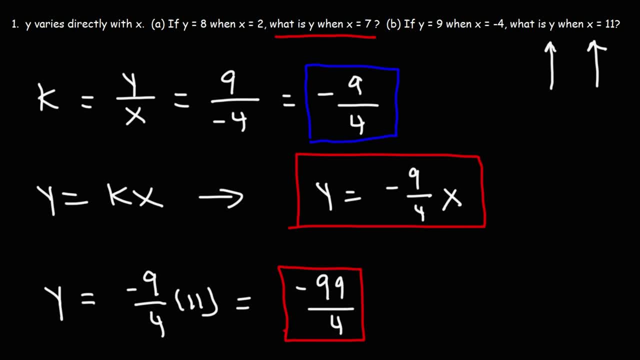 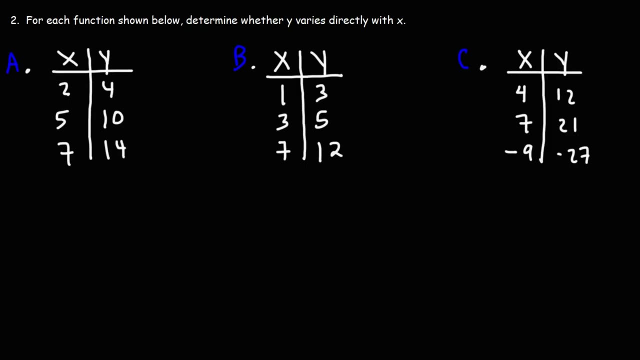 If you want the decimal equivalent of that, this is negative 24.75.. So that's how you can solve direct variation problems. By the way, for those of you who want more problems on direct variation, including inverse variation and even joint variation, 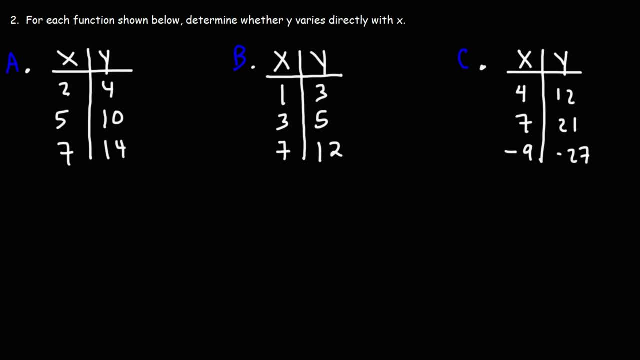 check out the links in the description section of this video. I'm going to be posting some other content there that you might find interesting. Now let's work on this problem. For each function shown below, determine whether y varies directly with x. So we're given the data in a table. How can we find the answer? 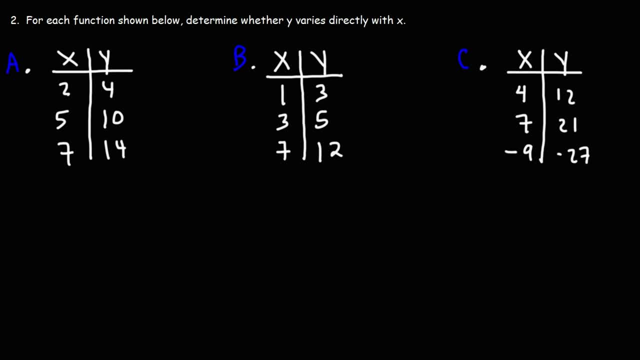 How can we determine if y varies directly with x? The key is to calculate the constant of variation. k is the constant of variation, k Keyword constant. For every pair of x and y values, k has to be the same. So remember: k is y divided by x. 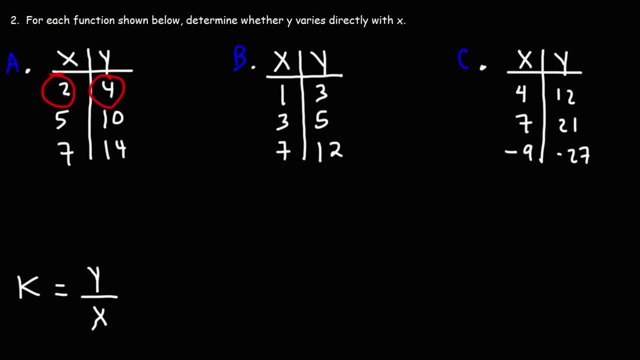 So if we take the y value and divide it by the x value, what do we get? 4 divided by 2 will give us k. So I'm just going to add another column for k. 4 divided by 2, we know it's 2.. 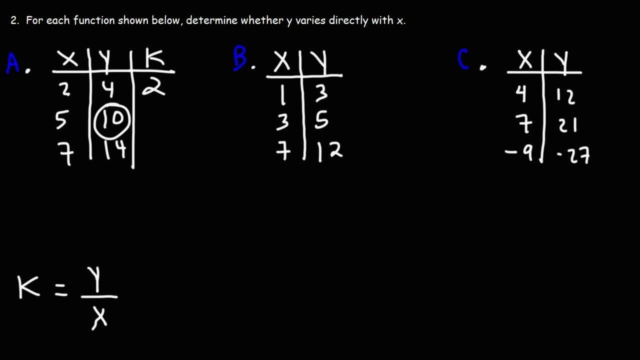 10 divided by 5 is 2.. 14 divided by 7 is 2.. So notice that k is constant. It doesn't change. So because it's constant, we can say yes For the first table. y varies directly with x. 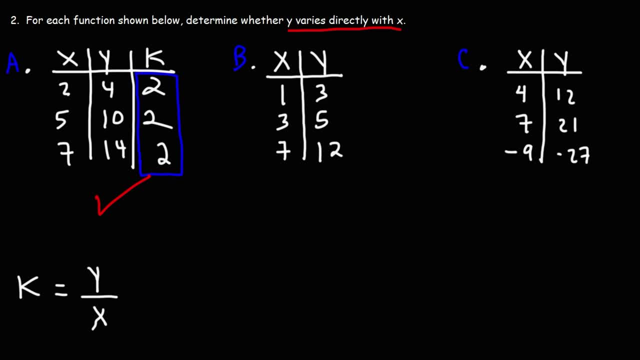 because we have a constant of variation. Now what about the second table associated with b? Let's calculate k for each pair of x and y values. 3 divided by 1 gives us 3.. 5 divided by 3, that's not 3.. 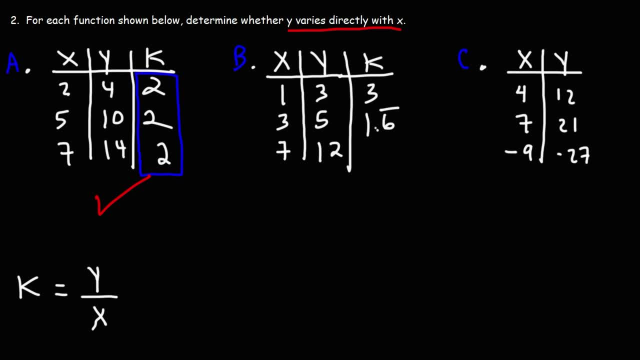 That's like 1.67 repeating or 1.6 repeating 12 divided by 7, that's not going to be 3 either. 12 divided by 7 is approximately 1.71.. So, looking at the values of k, they're not the same. 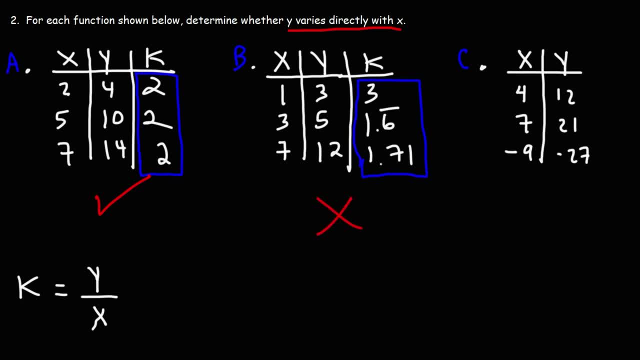 So we could say: y does not vary directly with x. Now let's move on to part c. Let's calculate k: 12 divided by 4 is 3.. 21 divided by 7 is 3.. Negative 27 divided by negative 9, that's also 3.. 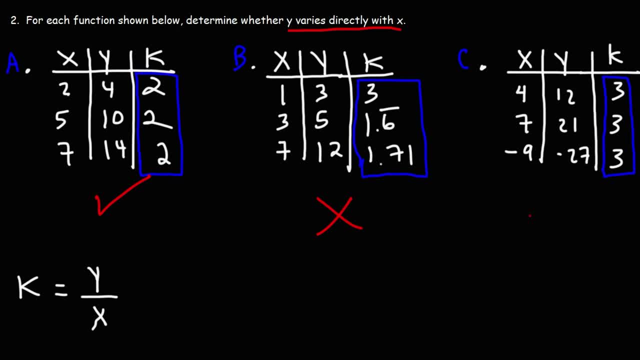 So for this table, k is constant, which means, yes, y varies directly with x. So that's how you could determine whether y varies directly with x or not. It's by calculating. Let me say that again, It's by calculating. 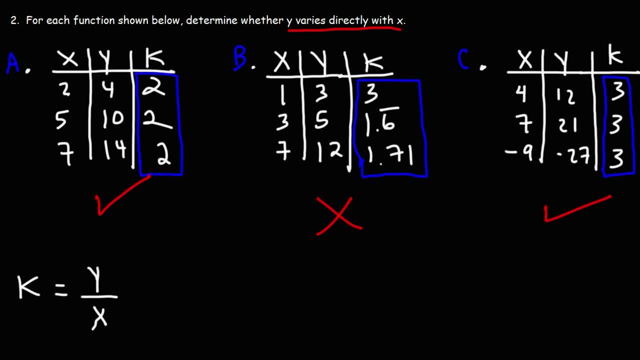 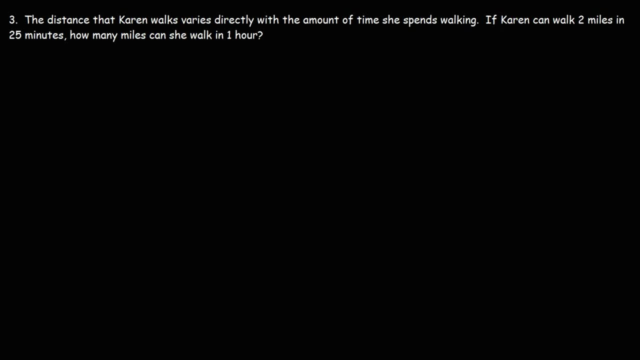 Number 3. The distance that Karen walks varies directly with the amount of time she spends walking. If Karen can walk 2 miles in 25 minutes, how many miles can she walk in 1 hour? So Go ahead and pause the video and try this problem. 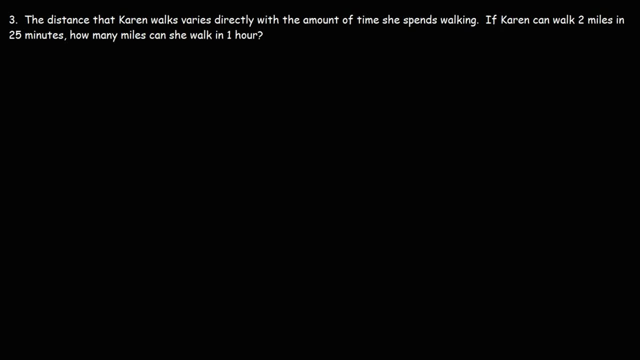 It's another direct variation problem. What we know is that the number of miles that she walks it varies directly with the time that she spends walking. So that is the minutes. So let's say y corresponds to the mileage And x corresponds to the time in minutes. 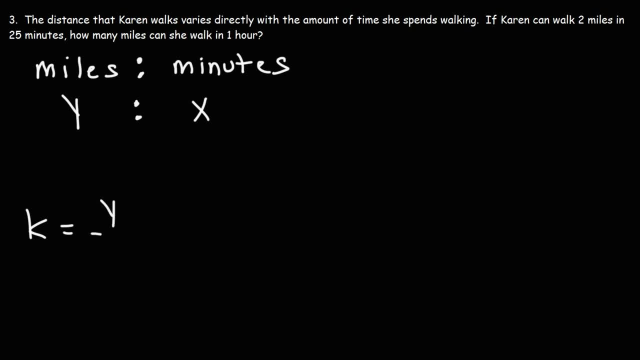 So we can calculate k. k is going to be y over x, So 2 miles for every 25 minutes, So k is going to be 2 over 25.. So that's step 1, finding the value of k. Step 2 is writing the equation. 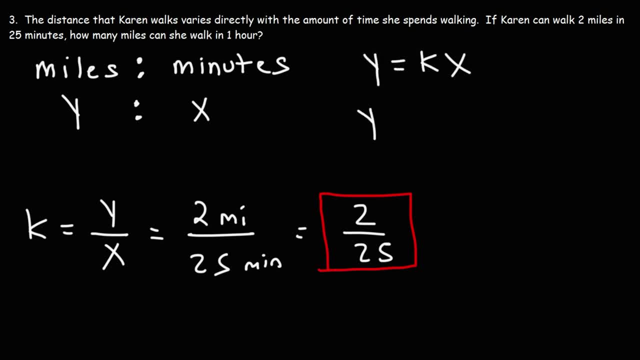 So y is equal to kx. Let's substitute k with what it is 2 over 25.. So this is the equation. Now x has to be in minutes. It can't be in hours. How many miles can she walk in 1 hour? 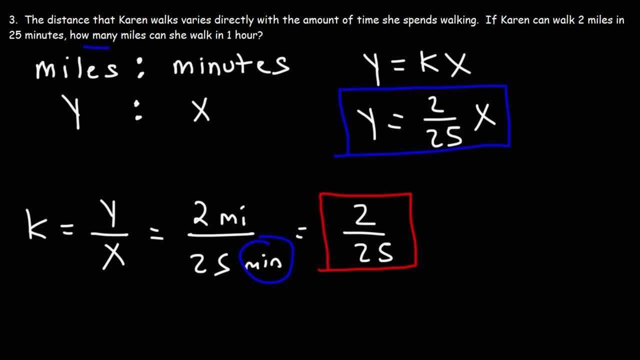 We need to convert hours to minutes. Fortunately, we know that 1 hour is equal to 60 minutes, So we can write the equation. So y is equal to kx. Let's substitute k with what it is: 2 over 25.. 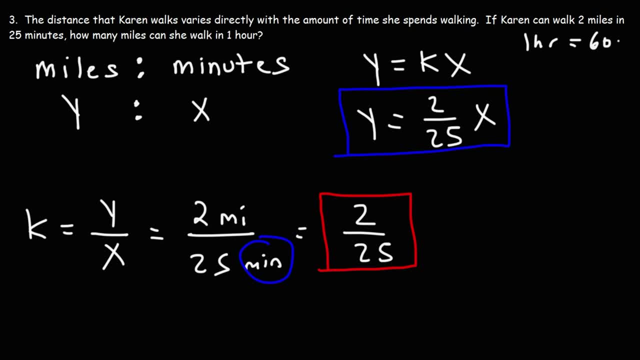 So this is the equation. Now x has to be in minutes. It can't be in hours, So all we need to do is plug in 60 into this equation And that is going to give us the mileage that she can walk in 1 hour.